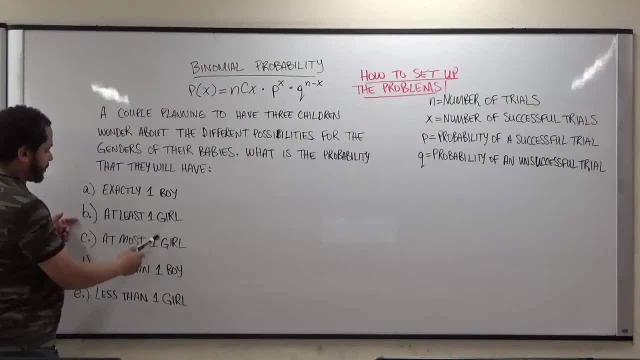 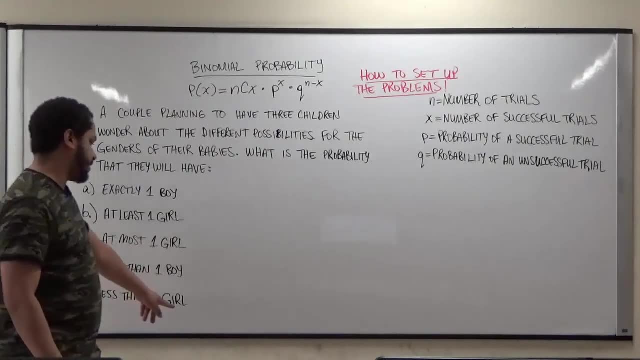 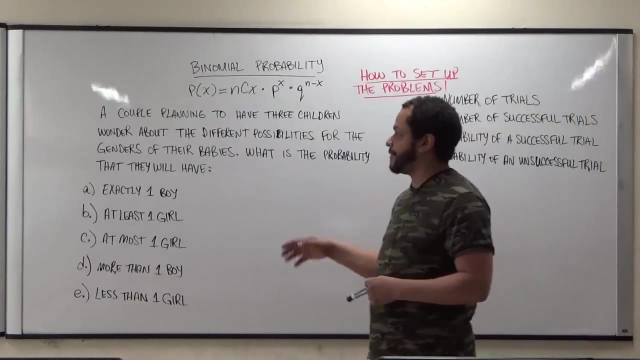 A- exactly one boy, B- at least one girl, B at most one girl, D- more than one boy and E- less than one girl. Now, before we can actually consider this to be a binomial probability distribution, we have to make sure it meets the four requirements, And for the first requirement, 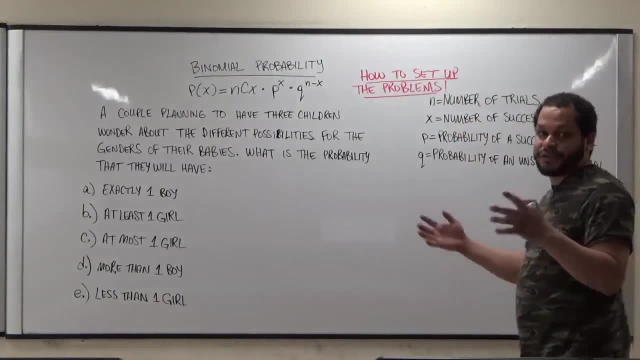 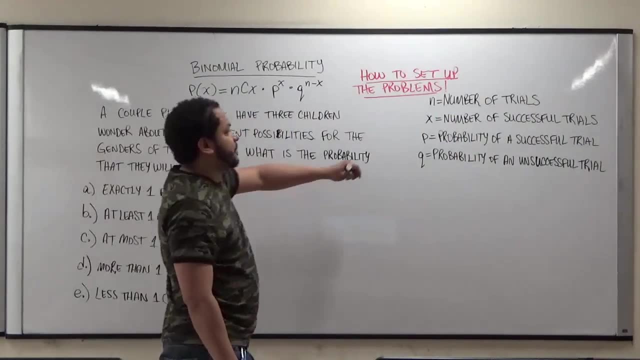 we have to make sure that this procedure has a fixed number of trials, Because we need to know the number of trials before we do anything And if you've seen the previous video, you'll know that the N, the X, the P and the Q are necessary components. 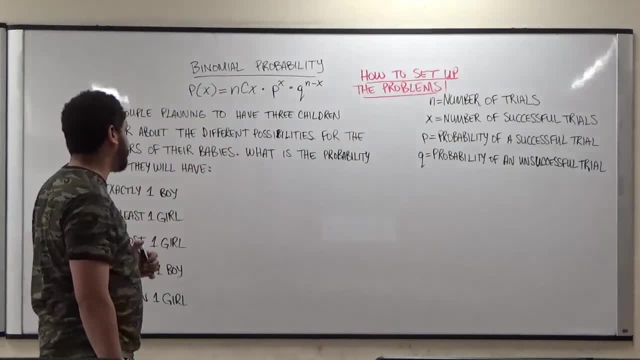 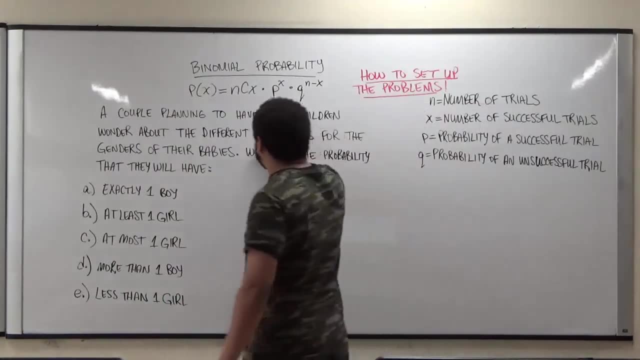 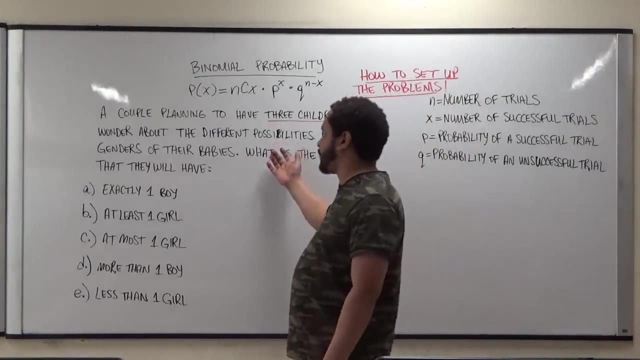 to determine whether or not it's a binomial probability distribution. Now, here, the fixed number of trials are the three children they're planning to have, And it's the three children because each child that they have is a trial of a different type of baby that they will. 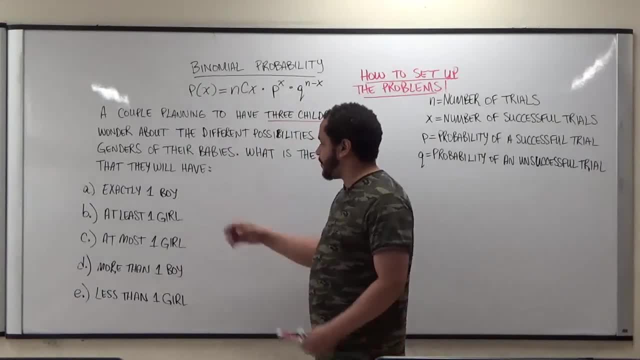 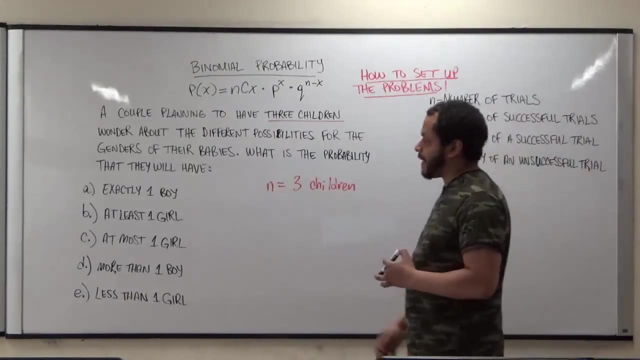 have Now. for each probability, the P and the Q will change, However, the N, the number of trials would remain to be three, because they're having three children. Now, the second thing that we need to know is that the trials are independent from one another, And here 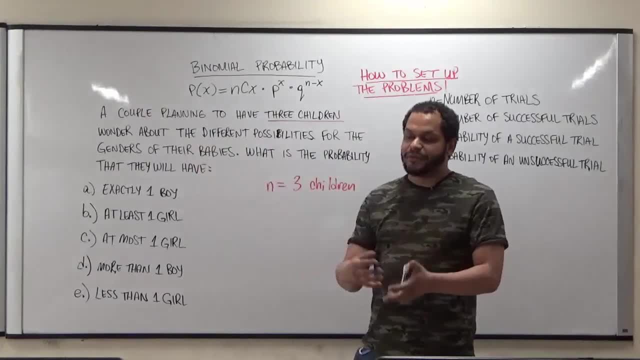 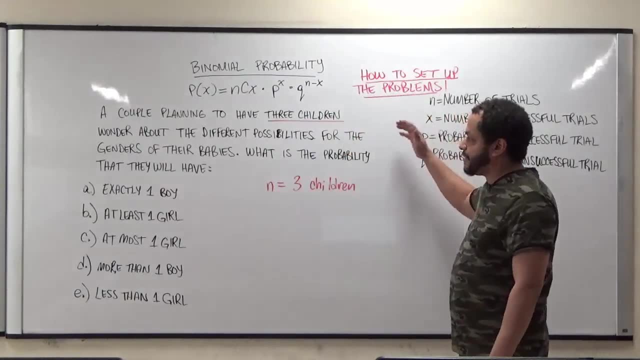 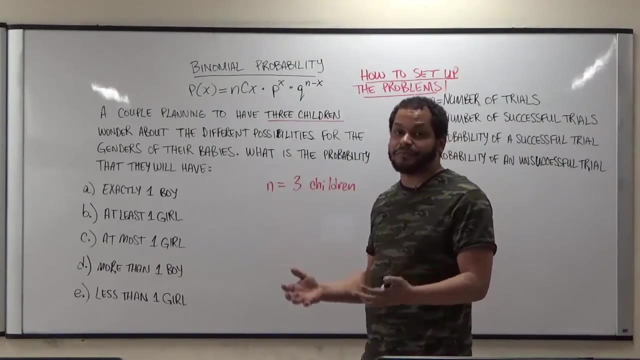 in every case of having a baby, this couple, their first child, would not affect the second child, would not affect the probability of the third child. So we know that the probability for each trial remains independent. If a couple has a boy first or a girl first, it doesn't affect which child will be born. 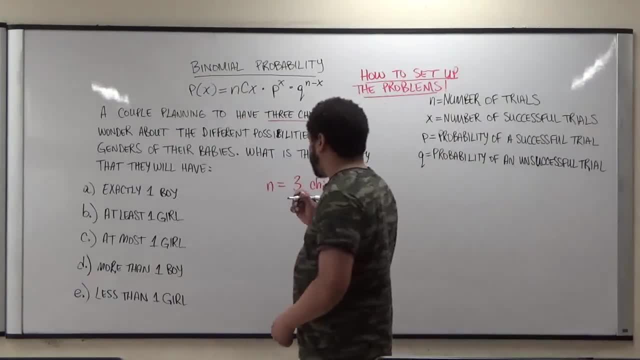 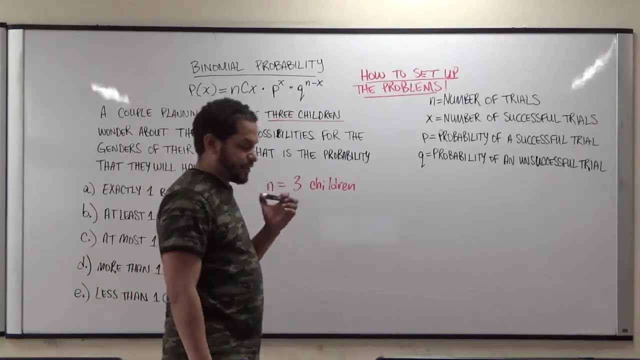 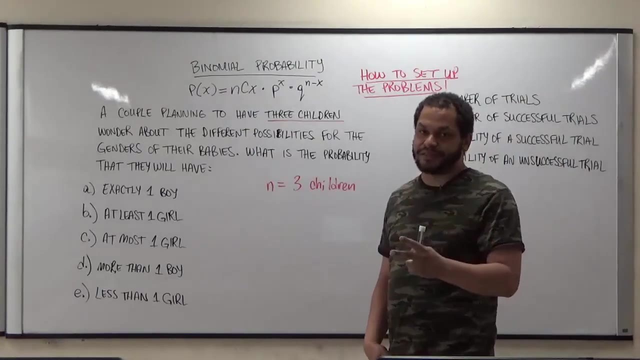 next. So we know that, then our probability for a successful trial in each case remains independent. Now, the third thing that we need to know for this is that each outcome is classified into two categories, specifically: right, And that's a success, or a failure, And that can. 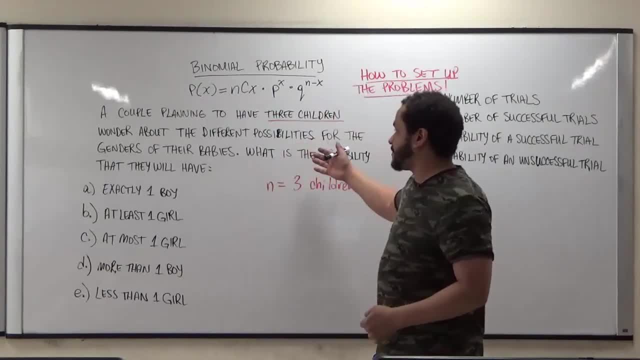 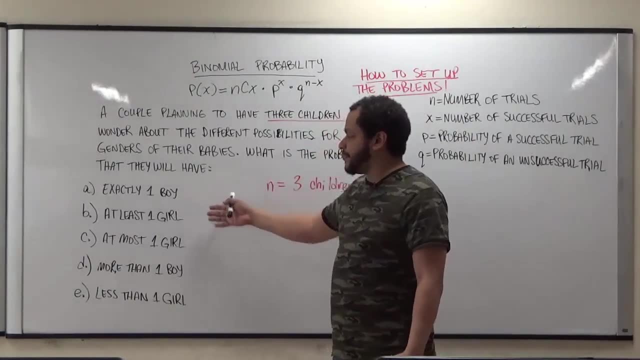 be like flipping a coin, getting a heads or tails Or, in this case, the probability of having a boy or a girl. So in the case we're looking at example A here- exactly one boy. the probability of a successful child would be one out of two. 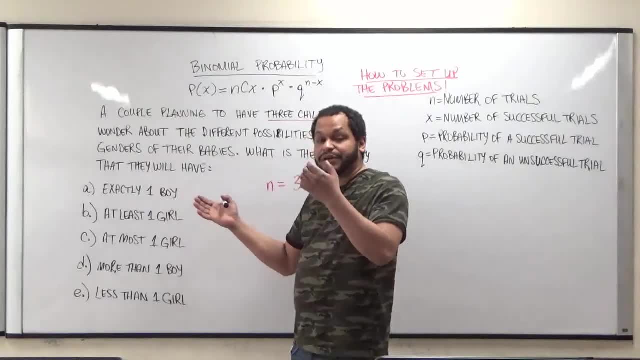 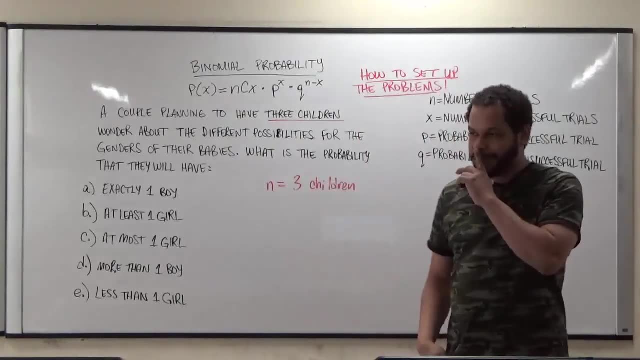 Whereas the probability of a failure for having a boy would be one out of two as well, because there's only two possibilities in having a child. So that checks off our third requirement. For the fourth requirement, we have to know that the probability for each trial or the 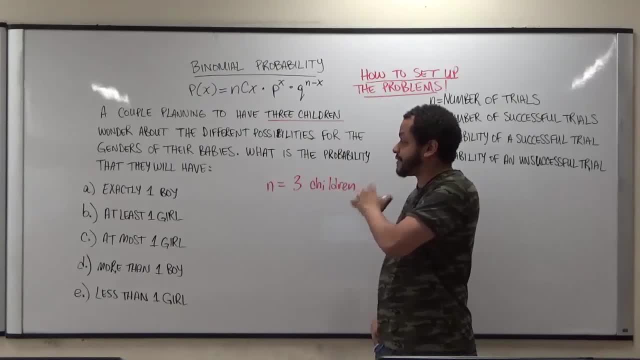 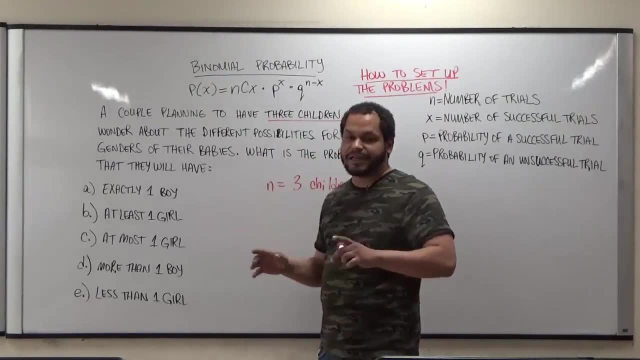 probability for each successful trial and every trial would be an even probability. That was because the probability of having a boy just measures the child as the success trial and every trial remains the same. and here again, because they're independent trials, we know that the probability of having a boy or a girl in that matter would not change for every event. 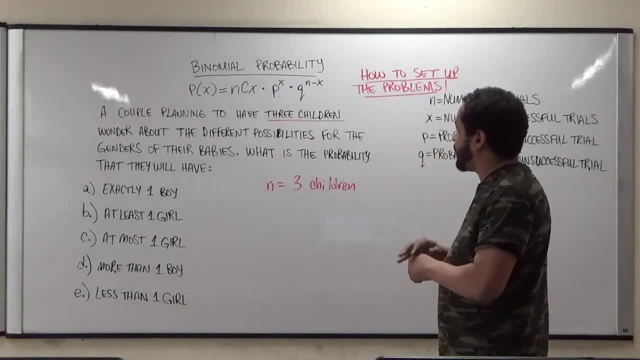 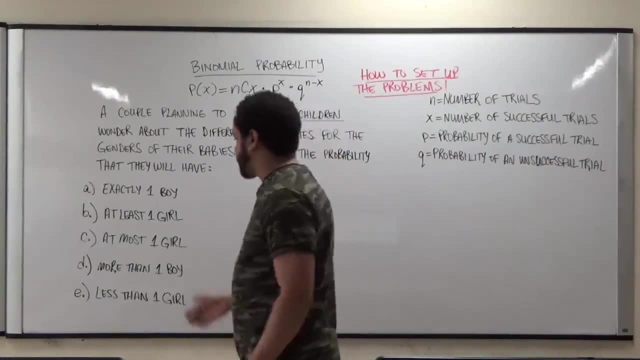 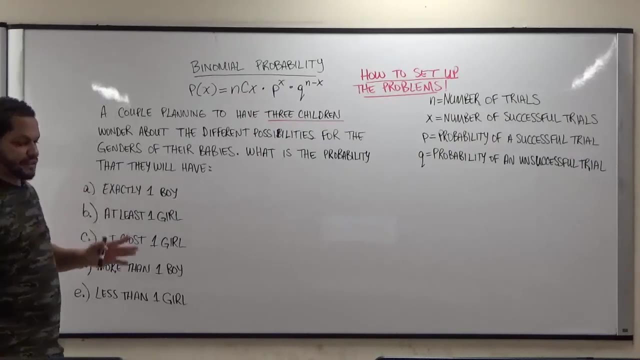 right, and so this makes this pass all the requirements for the binomial probability distribution. so let's begin with problem a. in problem a we have the probability of getting exactly one boy, b is again at least one girl, and c and so on, right. so what i want to do first is 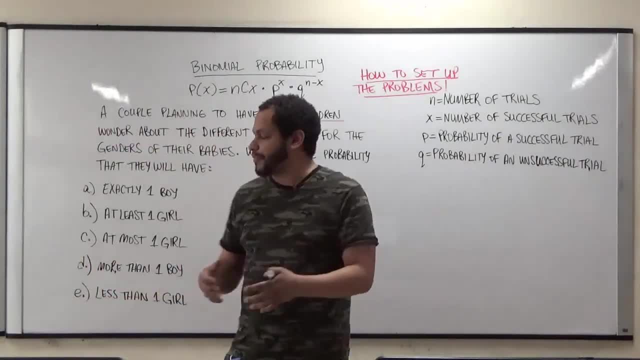 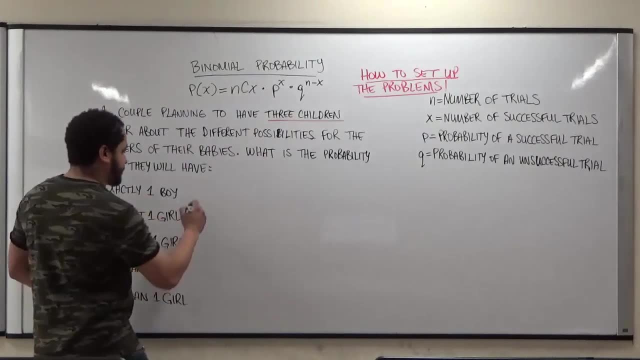 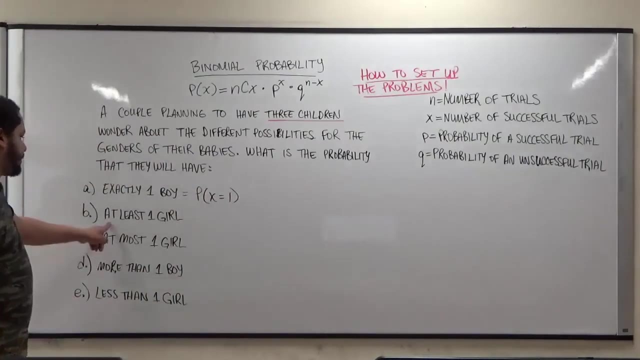 show you guys how to set up this problem so that you can begin your binomial probability distribution. for the first case, here we know it's asking us the probability of exactly one boy. so here we want to write: the p of x is equal to one. for this one it says the probability of at least. 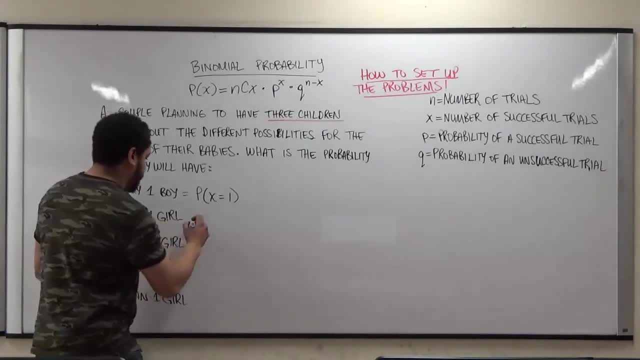 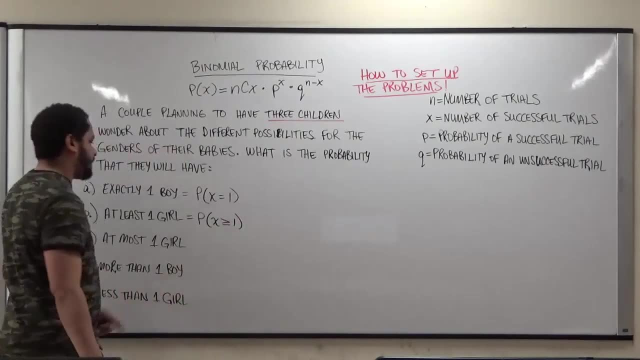 one girl, even though our p and q will be different for each one here this equation will become: the probability of x is greater or equal to one, and this is is. this goes all the way to the maximum number of trials. in this situation, our n is three, so it will go from one. 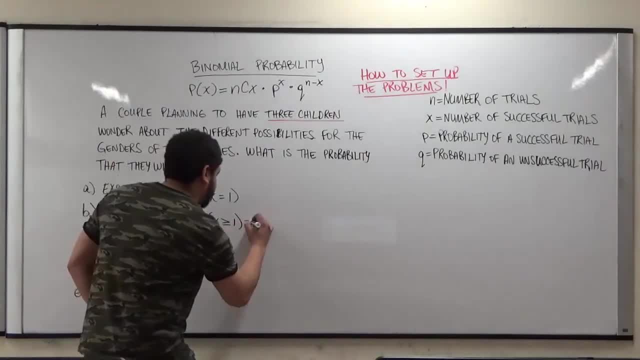 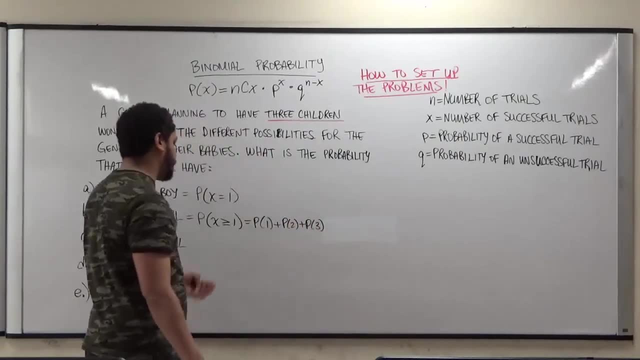 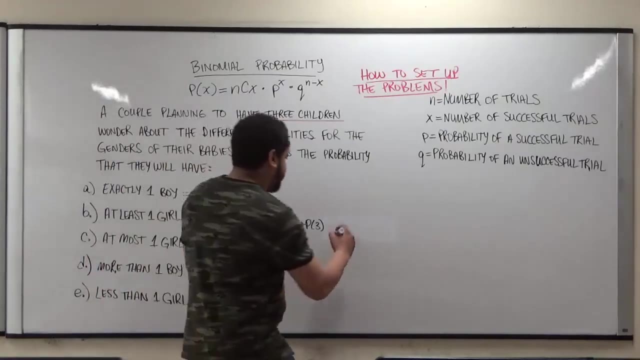 to two and three inclusively. right, so this will transform into the probability of one plus the probability of two plus the probability of three or, in a special case scenario where we're doing at least one, we subtract the probability of the zero case and we could say: this is either the 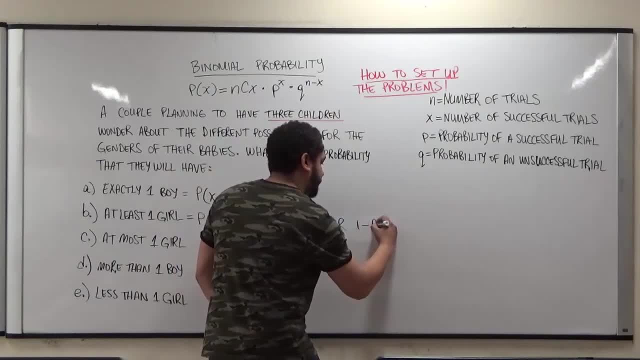 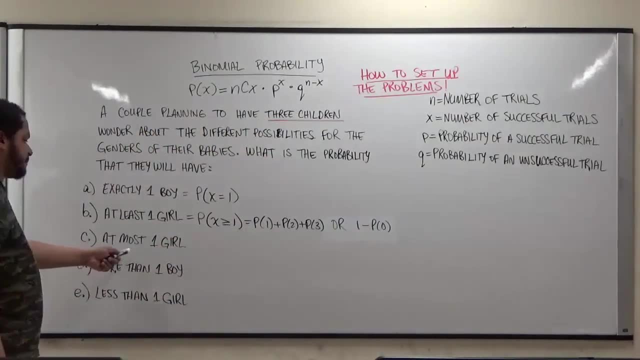 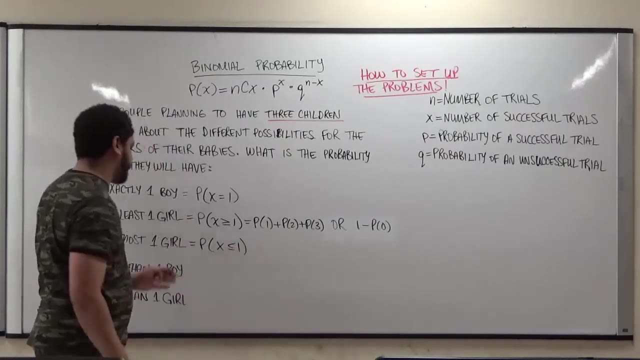 probability of one, two plus three or one minus the probability of zero, because it's the only case that doesn't have one or more. in the case of at most one girl, this is the probability that x is less than or equal to one, because it's one or less right, and so the probability for this situation would be the. 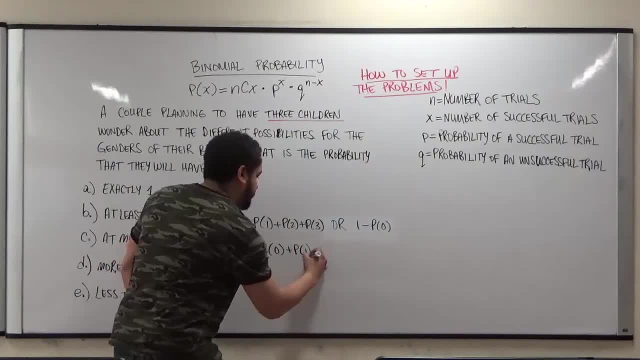 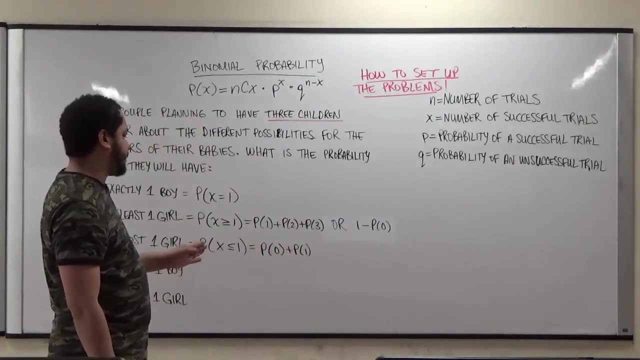 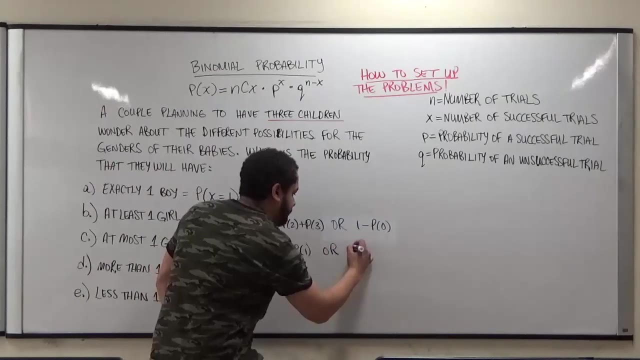 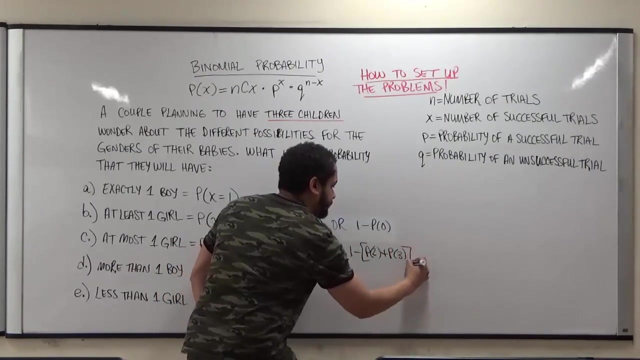 probability of zero plus the probability of one. another way that we could do this is similar to the at least one scenario is to subtract all the conditions that don't meet the at most one condition. So this would be this, or it would be: 1 minus the probability of 2 plus the probability of 3.. 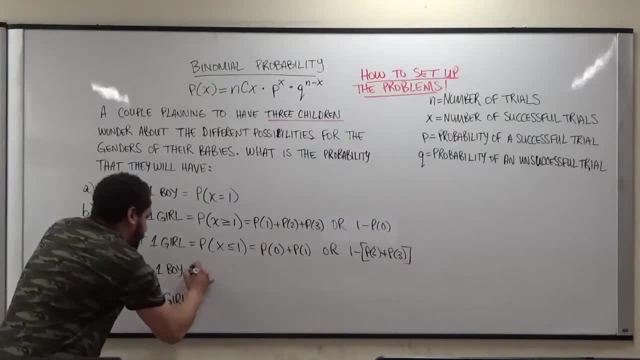 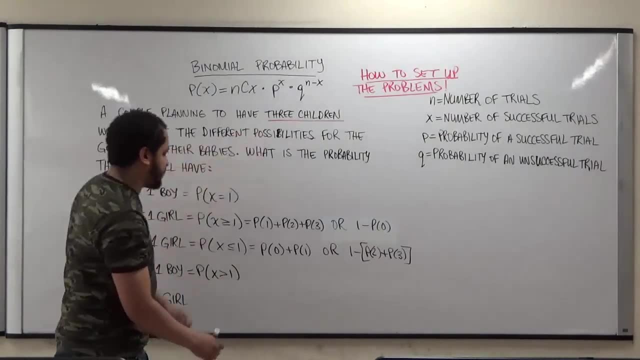 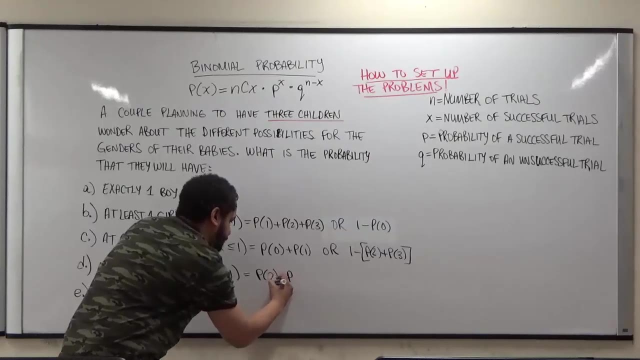 Now for the case of more than one boy. we'll have the probability that X is greater than 1. And in this case, because the maximum number of trials are 3,, we have the probability of 2 plus the probability of 3.. 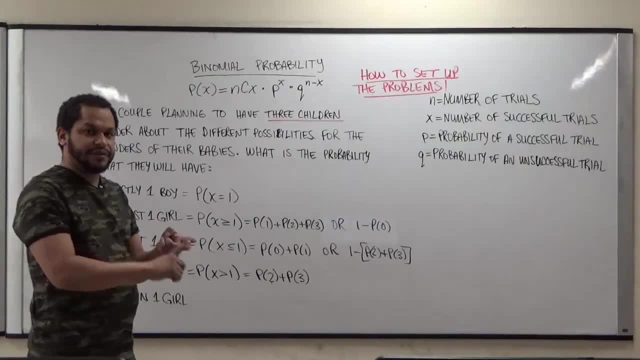 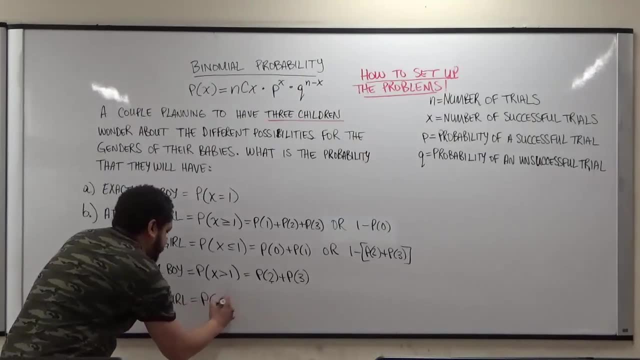 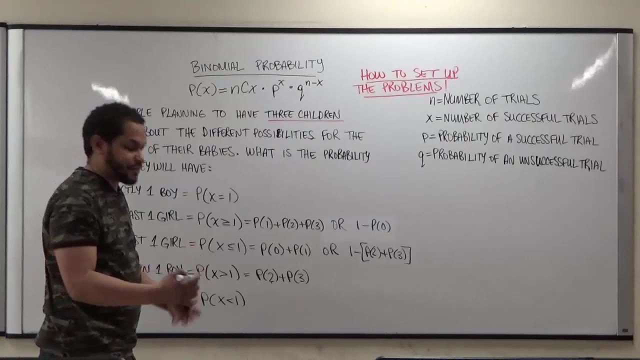 Because more than one boy would be having 2 boys or having 3 boys. Now, in the final case here, less than one girl, this will be the probability of X being less than 1.. And in this scenario, the only thing having less than one girl will be is having no girls, right? 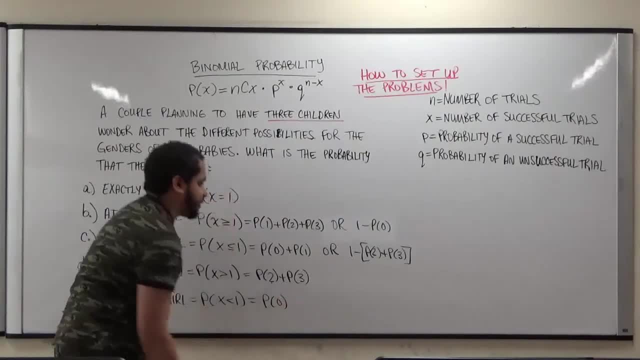 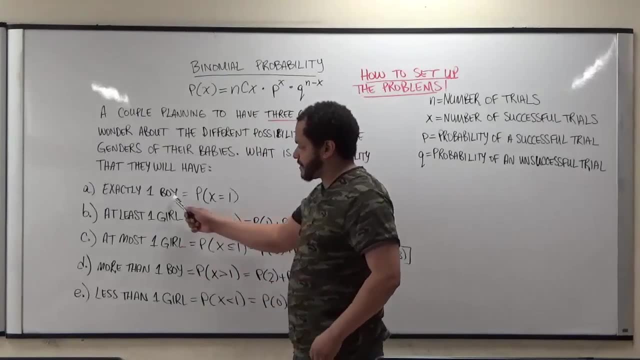 So this would be just the probability of 0 girls. Now, this is how we set up each problem, but for each problem we have to remember the situation of a successful trial being a boy or a successful trial being a girl would work in different ways. 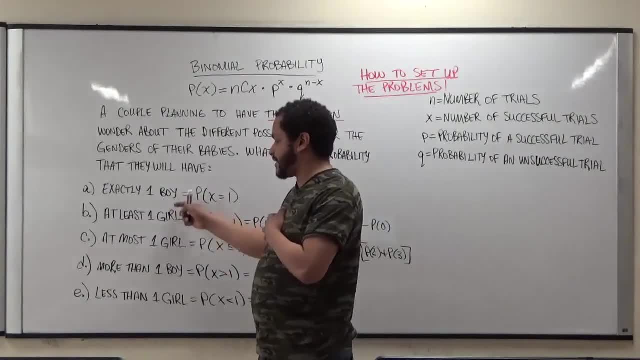 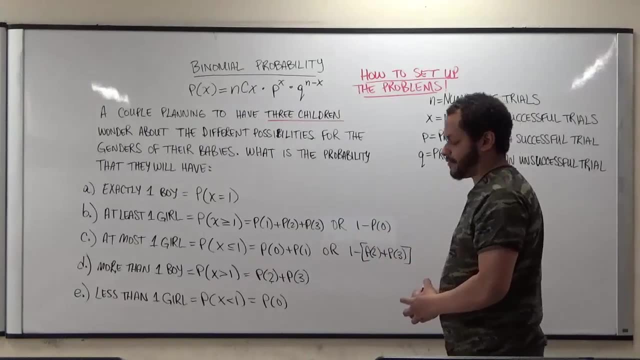 But, to our advantage, each of these probabilities of success are only 50%, So for that case, we can resolve each of these and still get the same result, regardless of which way we do it, Because our specific situation has a 50-50 chance. 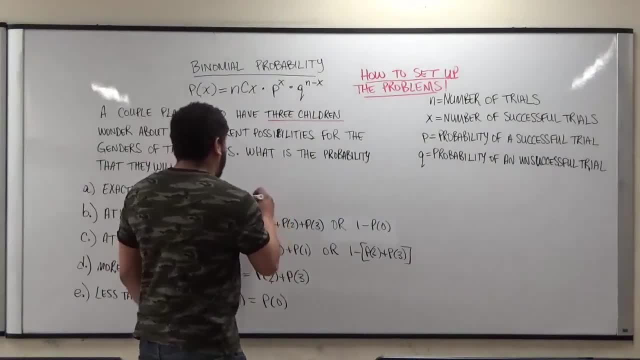 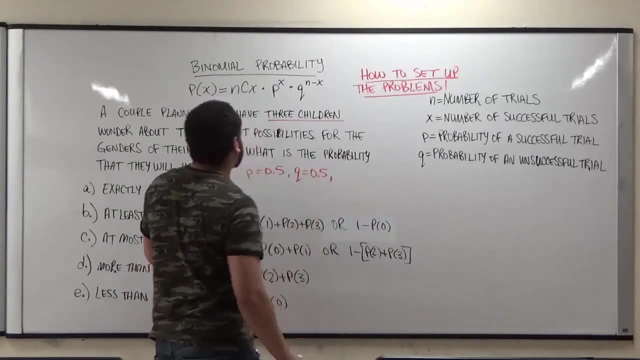 So let's begin with our first probability. So here we have. the probability of success here is 50%. The probability for not having a boy is Q, which is also just 50%. Our number of trials are 3 children, and it's 3.. 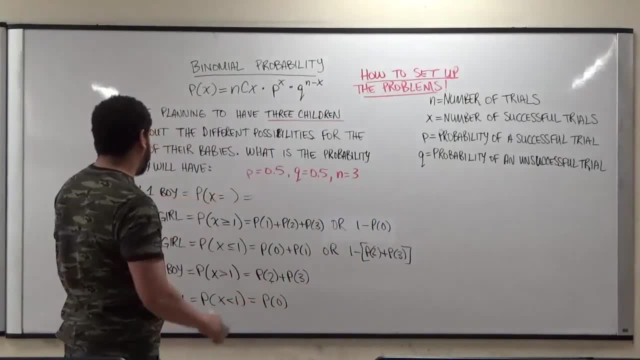 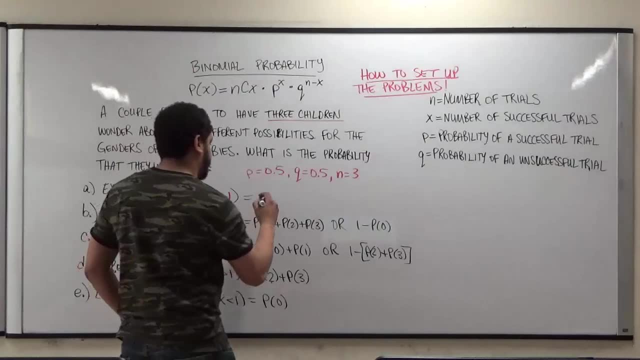 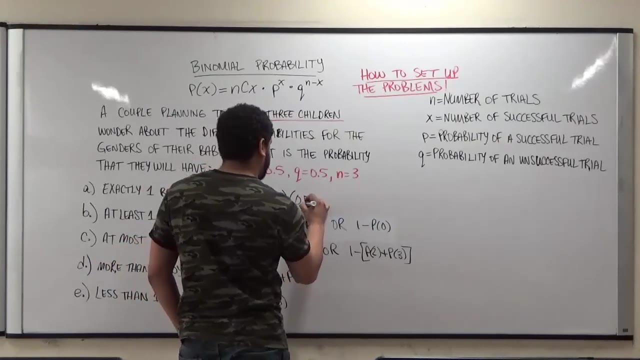 And in this particular case, our probability of successful trials would be exactly 1 boy. So here's where the 1 goes. So let's calculate this and set it up right. So we have 3 combination 1.. This is going to multiply by 0.5 times. 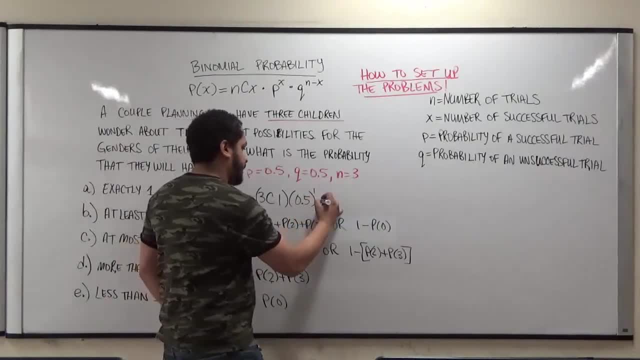 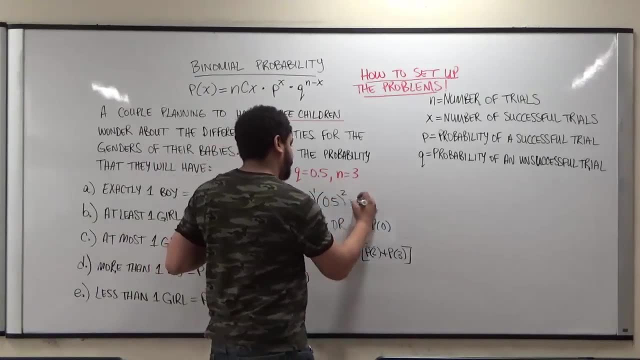 well, to the power of 1.. And that's multiplying by 0.5, which is Q, to the power of 3, take away 1, which is 2.. Right, 3 combination. 1 here is going to be 3, factorial. 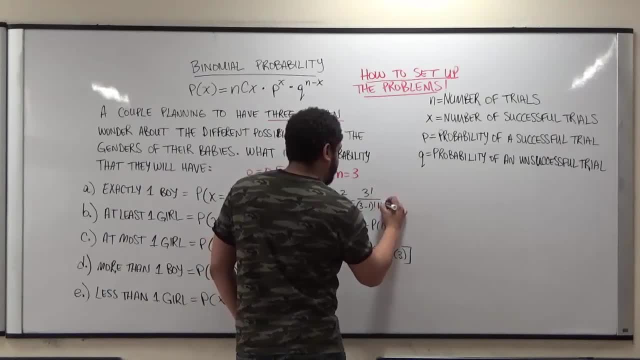 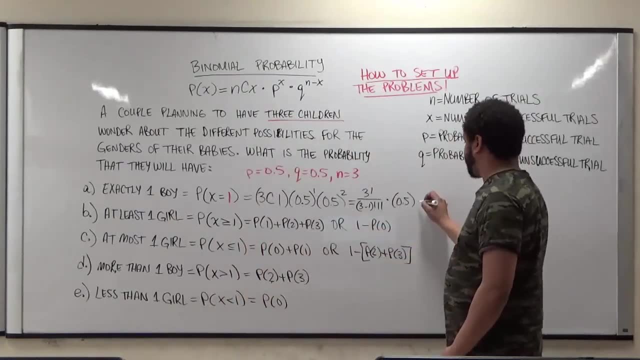 Over 3 minus 1.. Times 1 factorial. Times 0.5 to the first power is just 0.5.. 0.5 to the second power is 0.25.. And here we're going to have 3 factorial over 2 factorial. 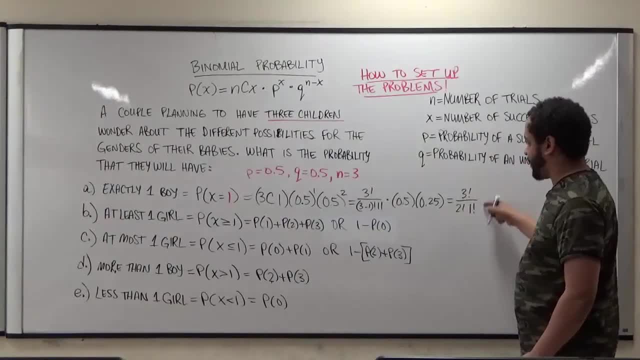 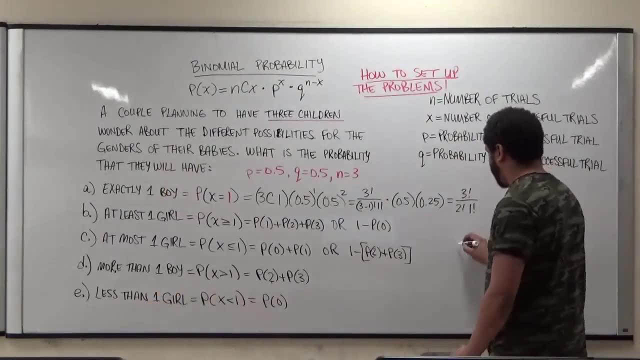 Times 1 factorial. And this, if we rewrite this, we know that this is 3 times 2 times 1, right? So here I'll just work this out on the side of it real quick. So we have 3 times 2 times 1 over, 2 times 1 times 1.. 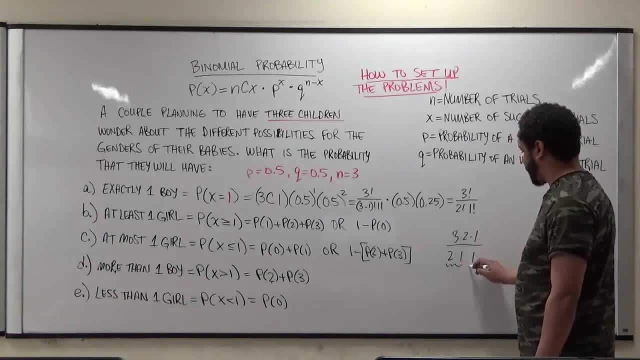 And this is the 2 factorial right here, This is the 1 factorial right here And this is the 3 factorial up top, And we notice that the 2 times 1 just goes away with the 2 times 1, and we just get a 3 for this result. 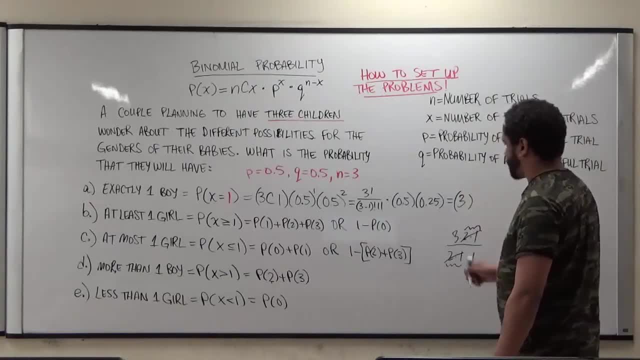 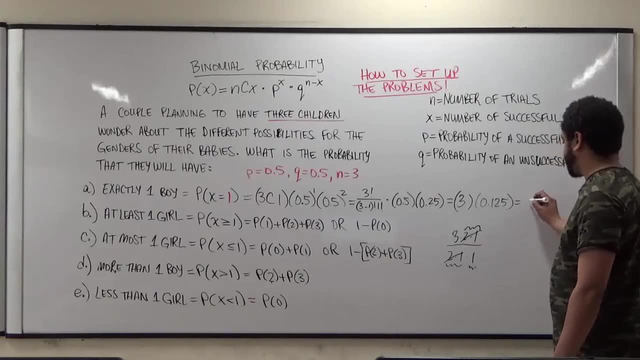 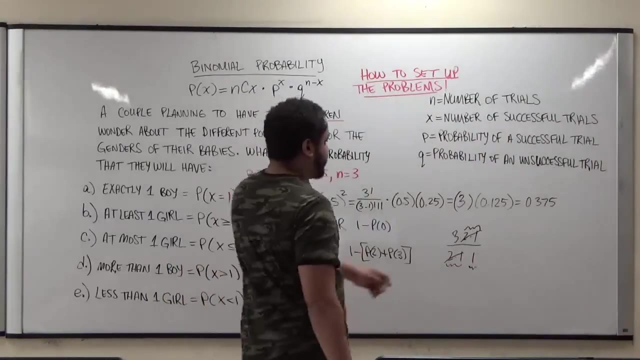 So we're going to have 3.. 0.5 times 0.25 is 0.125. And this then becomes 0.375.. So the probability of having exactly one boy is exactly 37.5% if we change this to a percent. 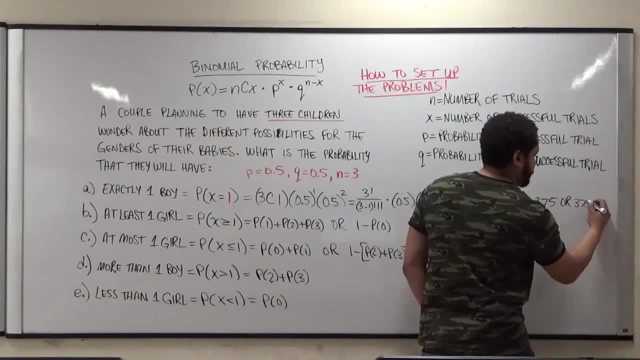 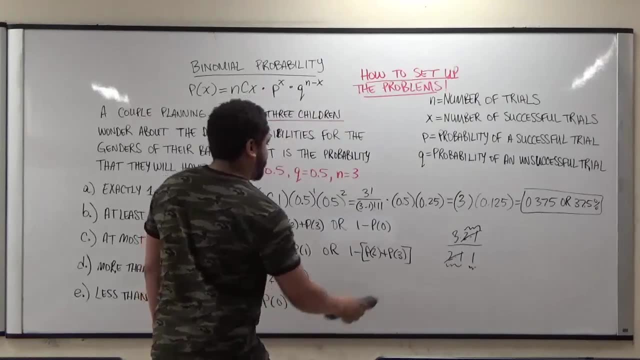 But we could keep this as a decimal as well, So either of these two solutions will do. Now let's move on to the next one. right, I'll wipe this down so we can continue with this one, And because this is a special case scenario. 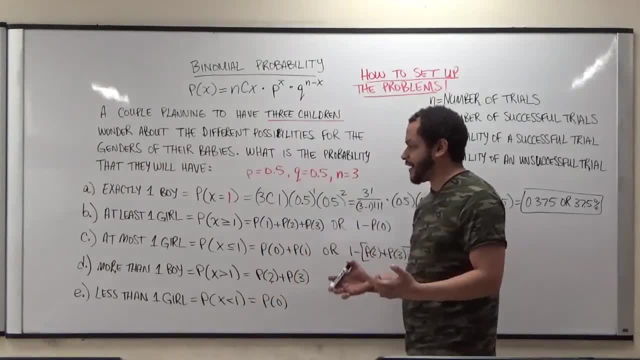 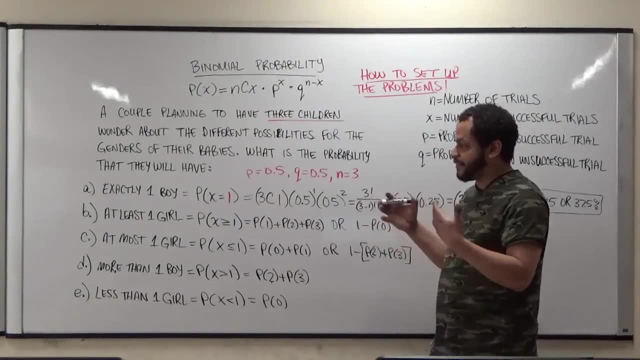 we recommend that most students- if you're doing the case of at least one- we use this condition, the complement event, which is one. take away the probability that they have no girls, right? So again, our probability of success for this trial is going to be 0.5. 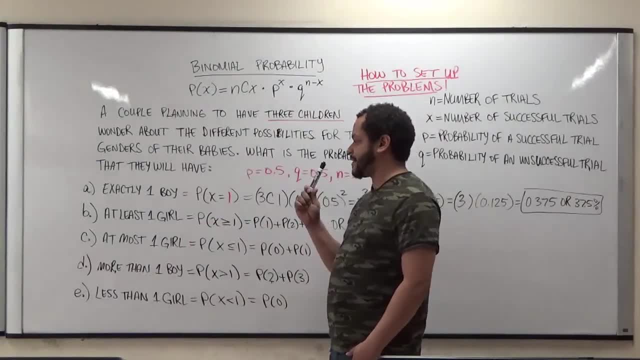 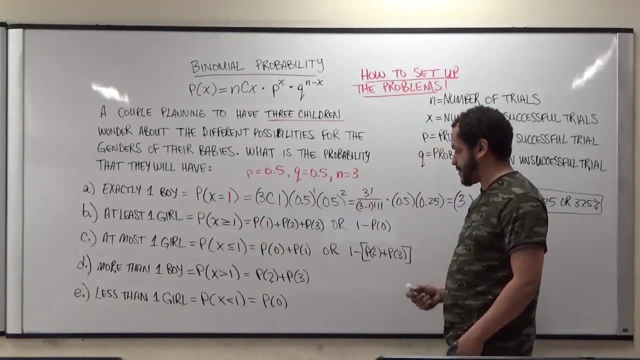 because the probability of getting a girl is exactly one half And the probability of not getting a girl is 0.5. again, The number of trials remain the same. It's 3 children for this couple. And to close out the probability, 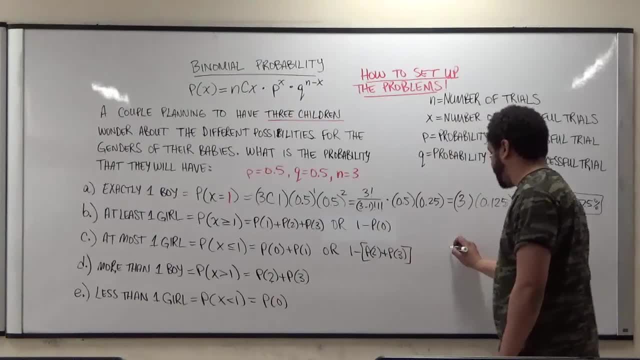 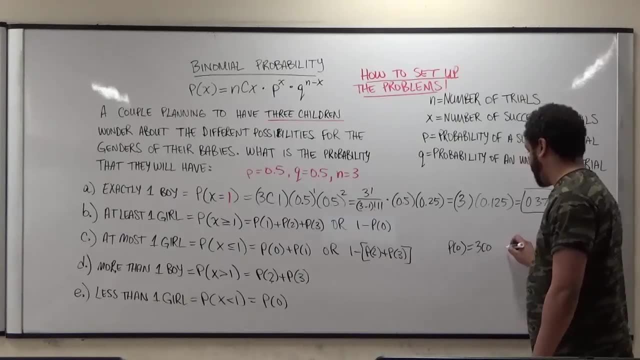 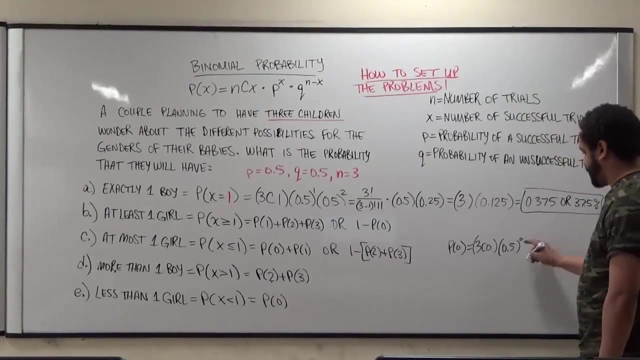 we just have to solve what the probability of 0 will be, the probability of having no girls. So here we have 3 combination 0. And we're multiplying that by 0.5 to the power of 0. This is a nice little function to use, because this becomes 1.. 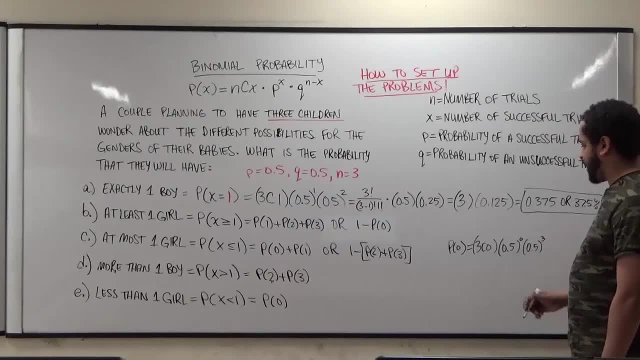 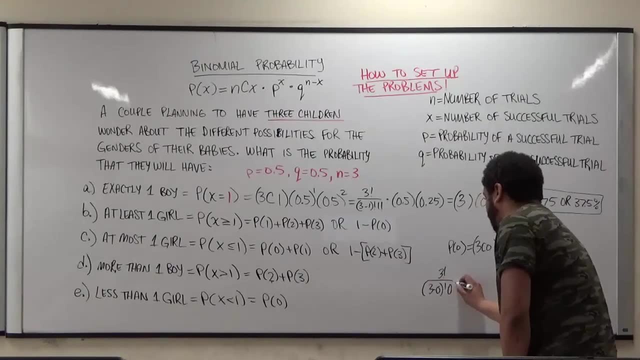 And then we have 0.5 to the third power, And so 3 combination 0,. let's inspect what happens. We have 3 factorial over 3 minus 0 times 0 factorial And a good little pop quiz. Whenever you get 0 factorial, this becomes 1.. 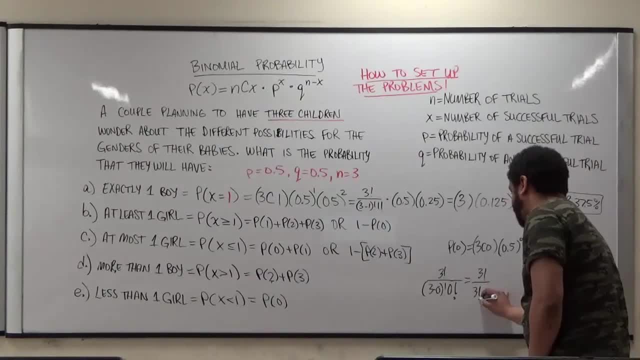 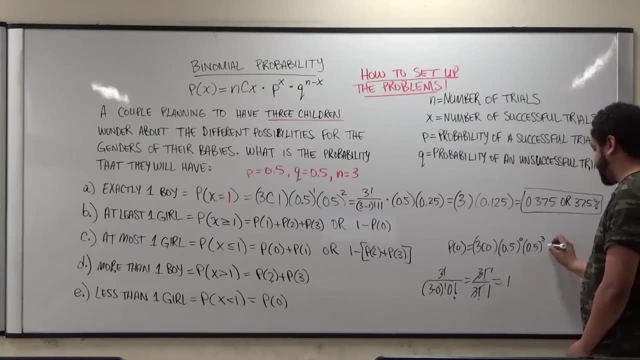 So we have 3 factorial over 3 factorial times 1.. The 3 factorial is reduced to 1 exactly and we get 1.. So 3 combination 0 is just 1.. And then we have 0.5 to the power of 0 is 1.. 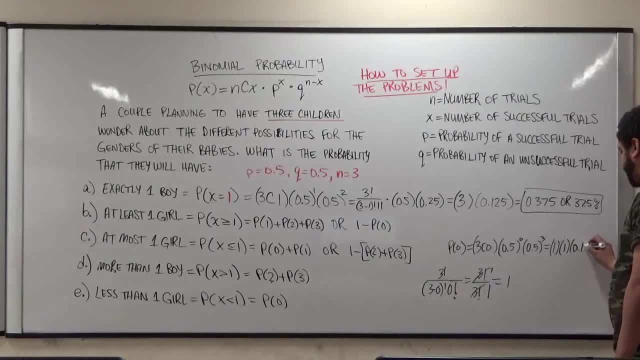 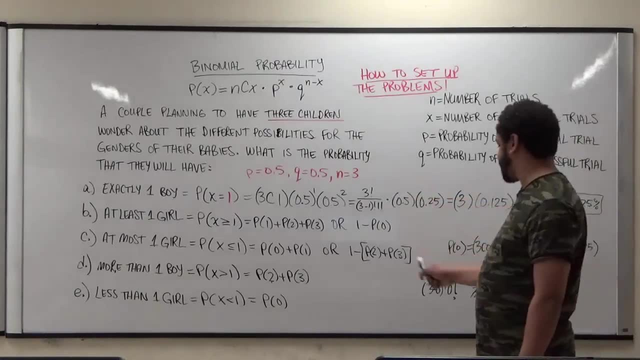 0.5 to the power of 3 is 0.125.. And so the probability of having a 0 or no girls out of 3 children is going to be 0.125.. And here we just have to complete that formula. 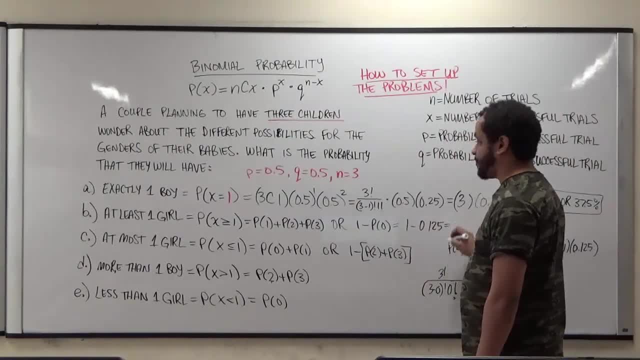 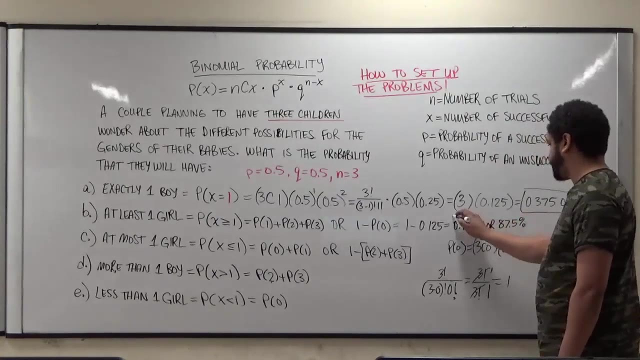 We have 1 minus 0.125.. And the probability of having at least 1 girl and 3 children would be 0.875 or 87.5%. Either of these 2 answers will do. Make sure that when you have your decimal to get the percentage. 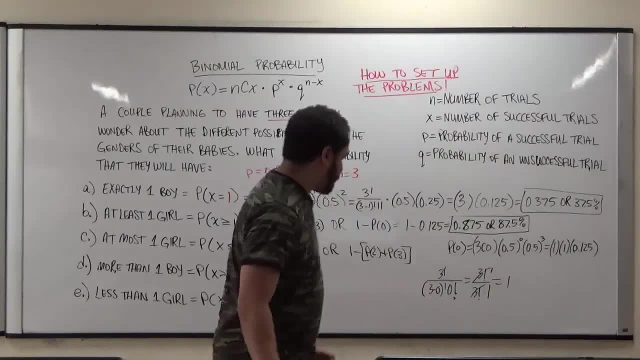 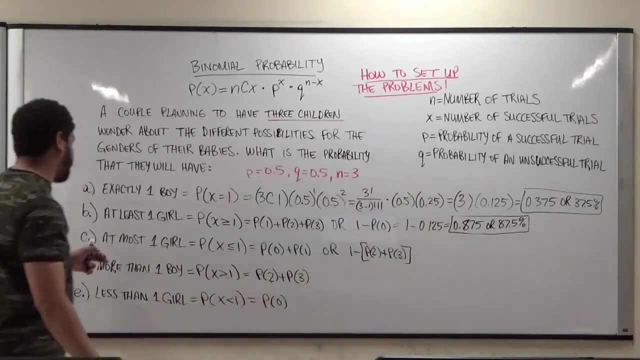 you multiply this decimal by 100%. Let's move on to the next piece. I'll wipe off this here. Make sure you're taking notes of this if you're watching the video. Now to get to the at most 1 girl scenario. 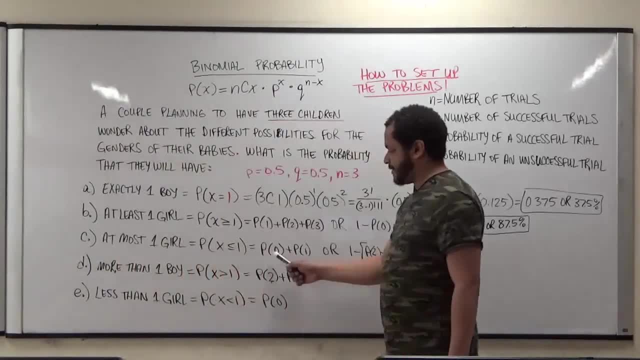 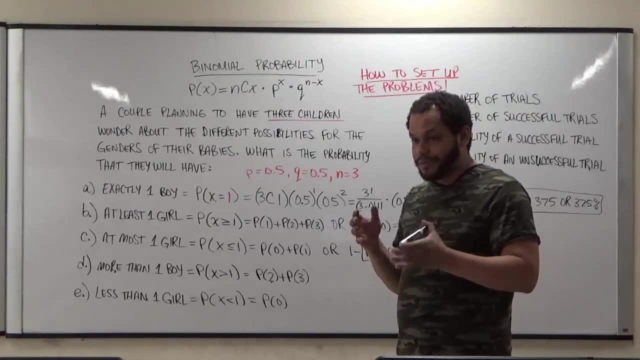 it doesn't really matter which one of these 2 we use, Because, to be honest, adding up 2 probabilities or taking 2 probabilities and subtracting them from 1 give us the same situation. We recommend that when you're doing this, 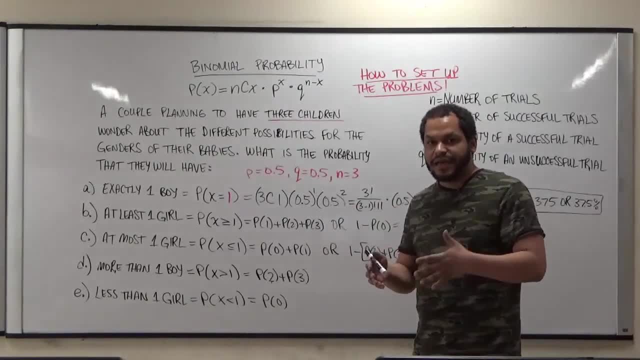 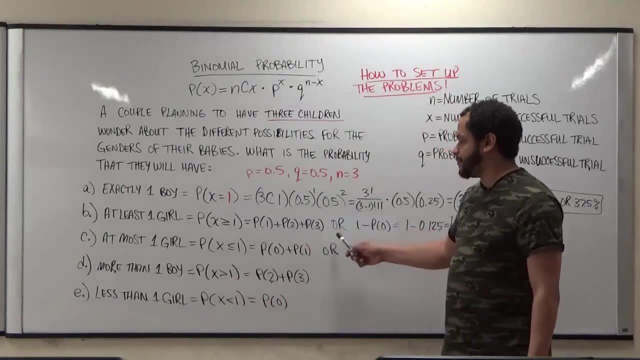 you look at which scenario is going to make you work less or work more, and consider it when you're choosing which way you want to work this out. The same goes for the at least principle. Sometimes it's not always going to be 1.. 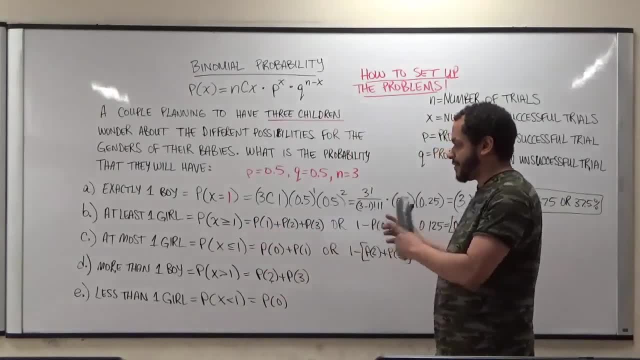 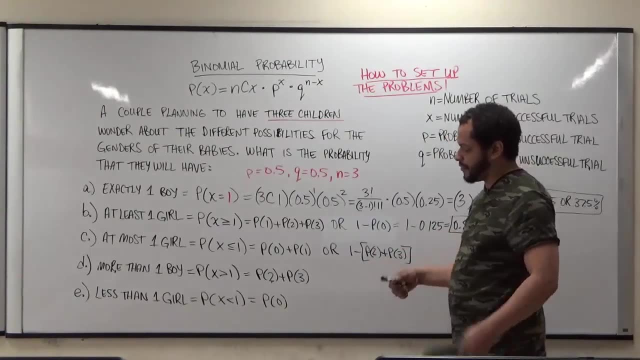 Sometimes it may be 3, and then you're going to end up doing more work. Make sure you weigh out the differences, because here I only had to solve 1 probability. Here I would have to solve 2 probabilities and subtract them from 1.. 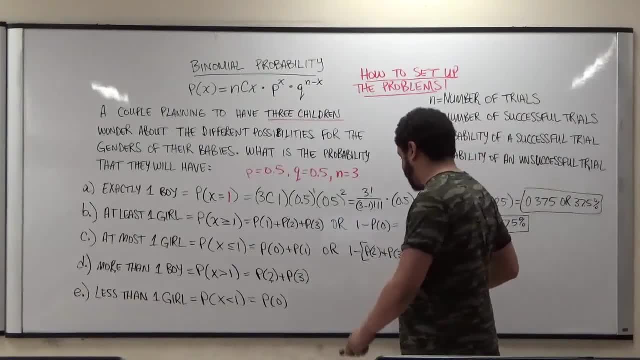 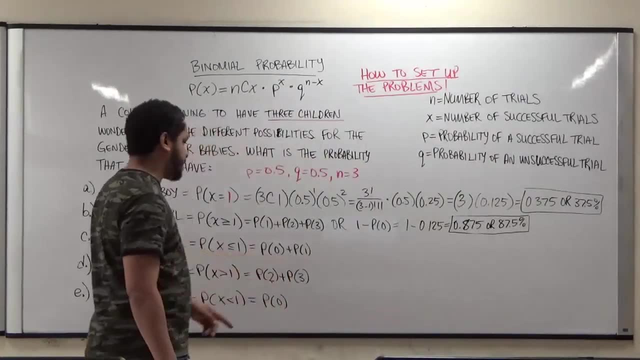 This makes 1 extra calculation that I pretty much would say I don't need to do right now, because it's the same as just adding 2 probabilities up Now. as far as the P of 0 goes, we did use this for the last problem. 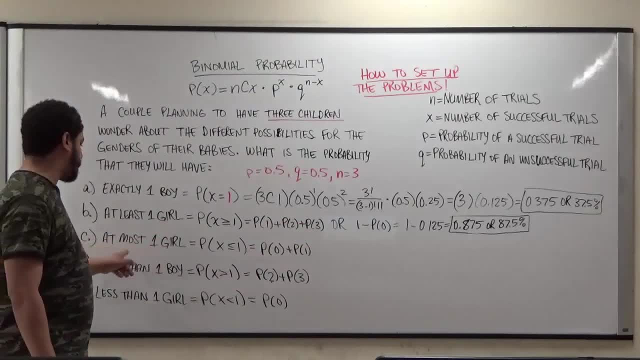 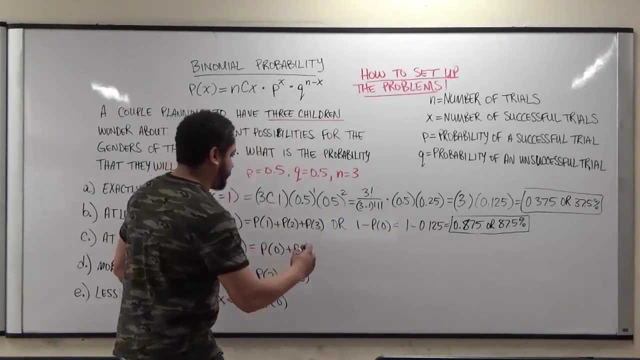 because here we're dealing with the same successful trial, which is a girl, And so the probability of at most 1 girl. we already have the 0, which is 0.125, done from the previous problem, So I incorporate that into this problem, again 0.125.. 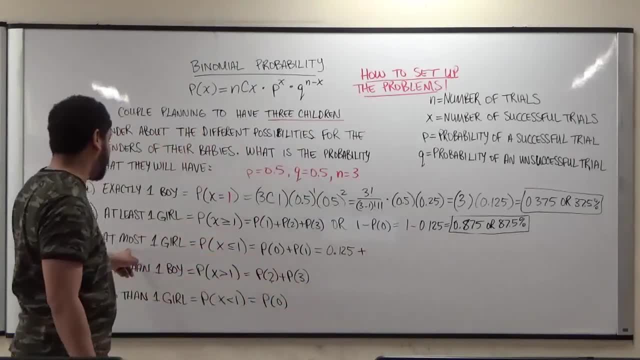 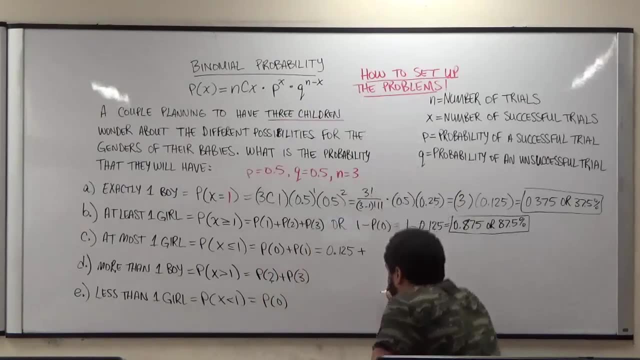 And to this we're adding the probability of having exactly 1 girl, because at most 1 girl is the probability of 0 plus the probability of 1.. So let's investigate what happens at the probability of 1.. And this becomes 3 combination 1. 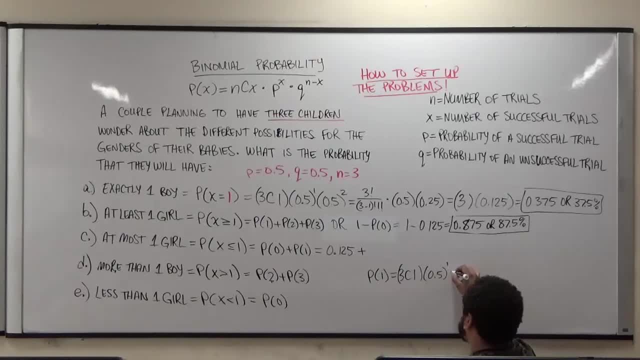 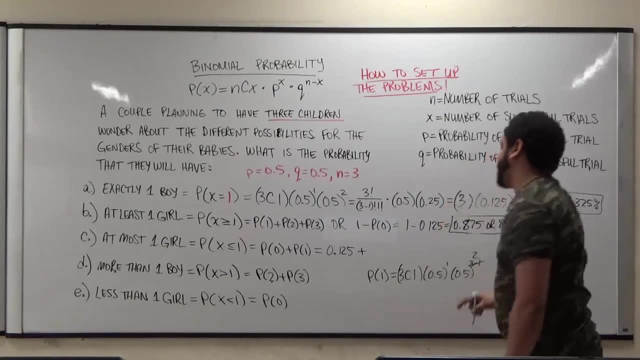 times 0.5, to the power of 1 times 0.5, to the power of 3 minus 1, which just becomes 2,. right Now, this is the same exact problem we did for the boy situation, even though it's not the same. 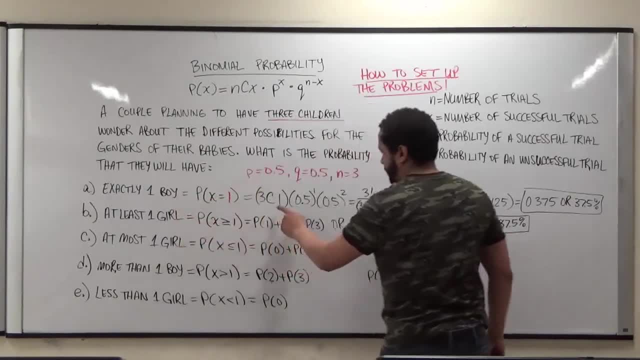 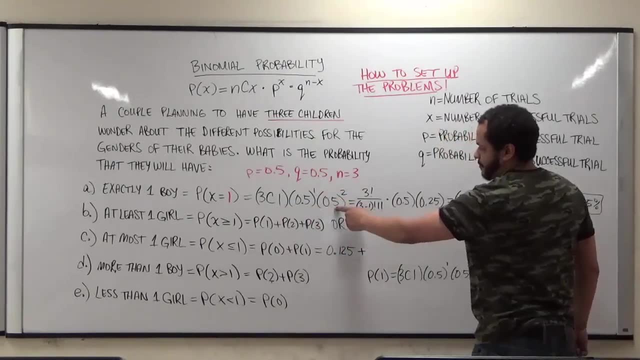 outcome that we're looking for with a boy and a girl, But the probability numbers are exactly the same. We have the 3 combination: 1,, 0.5 to the power of 1, and 0.5 to the power of 2. 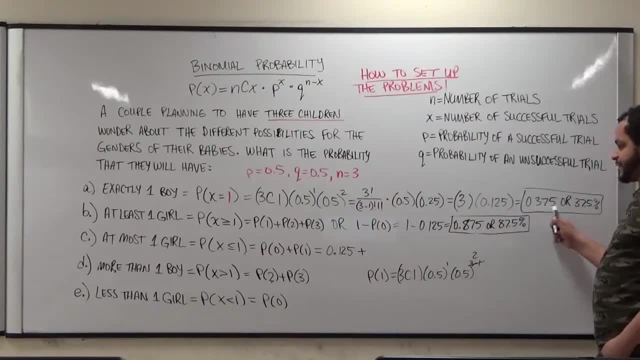 which we know came out to be 0.375.. So we're going to add this as the probability of 1, because this final result is 0.375.. We're going to add this to 0.125 now And when we add these 2 up. 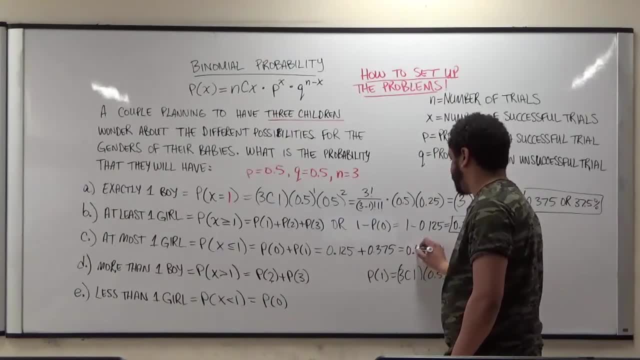 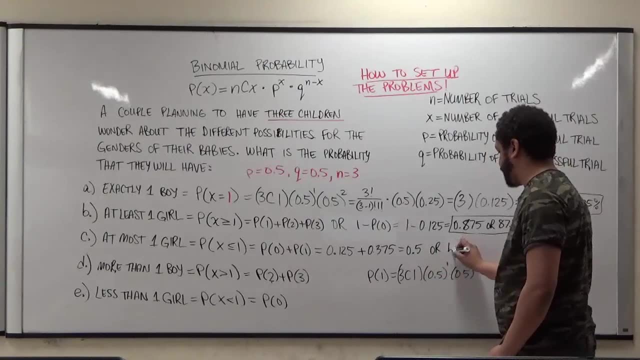 we get exactly 50%. So it'll be 0.5, or multiplying 0.5 by 100%, we get 50%, And that takes care of the answer for part C. Now, moving along, we get to the last 2 here. 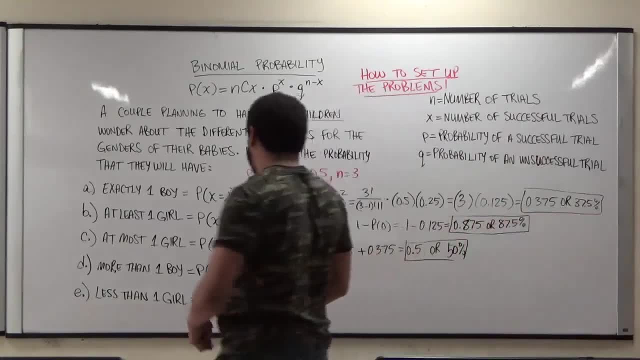 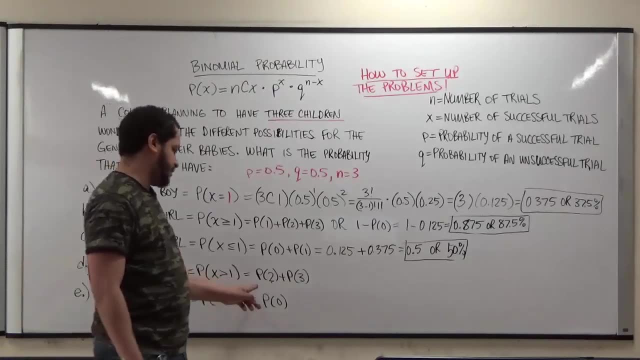 And in this case we have more than 1 boy and we can't avoid finding the probability of 2 and 3.. Because here we have, the p of x is greater than 1.. Greater than 1 would be 2 boys and 3 boys. right. 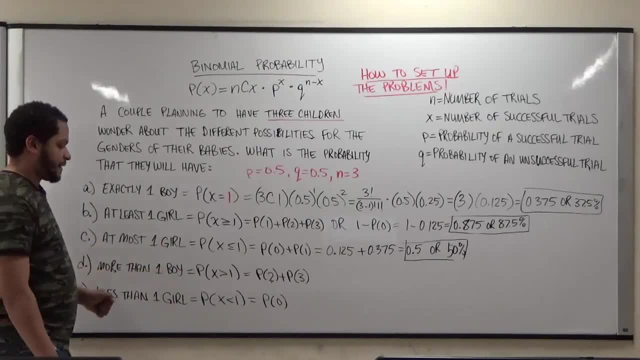 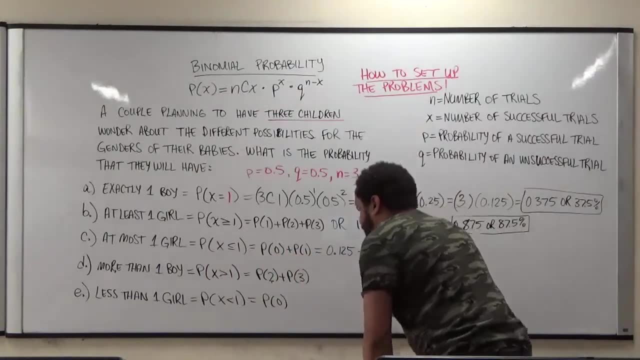 Because we're dealing with the situation of more than 1 boy. So in this case we have to resolve the probability of 2 and the probability of 3 separately, right? So let's get to it. So the probability of 2 boys. 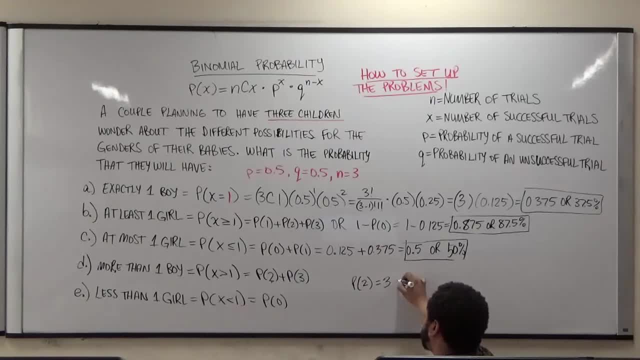 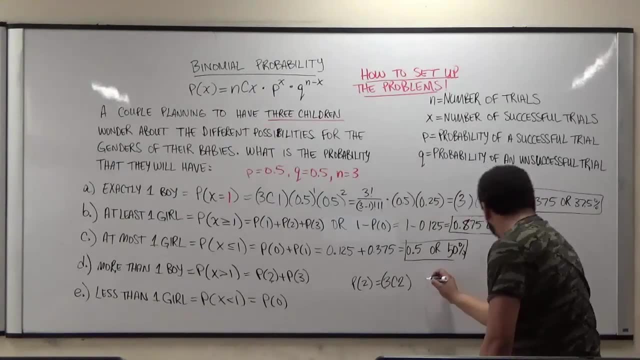 again will give us. the number of trials are still 3.. We have 3 combination: 2.. We're multiplying this by. We have here 0.5 raised to the power of nx, which is 2.. And here we have 0.5, right. 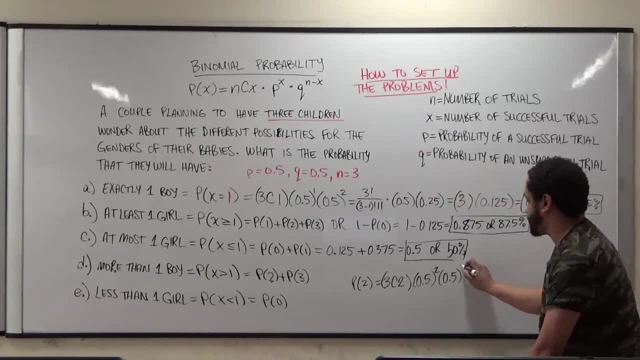 Right off of the formula raised to the power of n minus x, which is 3, take away 2. And this becomes the power of 1.. So now 3 combination 2,. let's take a look at the factorials here. 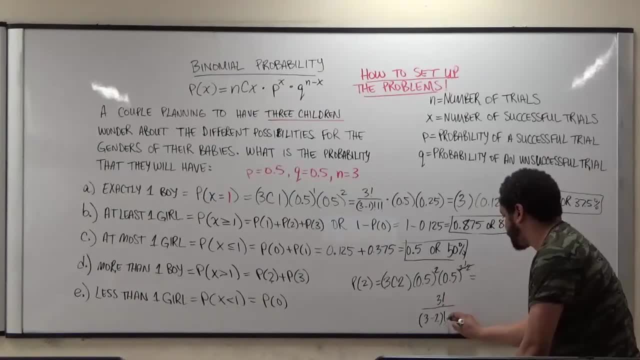 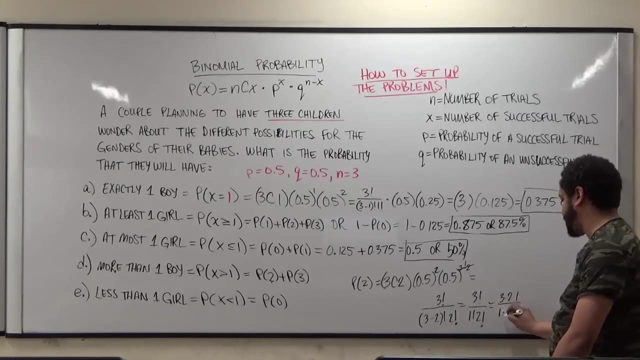 3 factorial. 3 minus 2 factorial times 2 factorial. This becomes 3 factorial over 1 factorial times 2 factorial. This becomes 3 times 2 times 1, right And on the bottom we have 1 times. 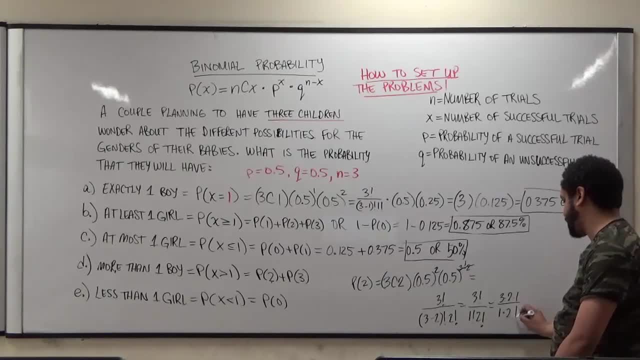 The 1 factorial is 1.. The 2 factorial is 2 times 1.. The 2 times 1 goes away and this just becomes 3.. So we have 3 multiplied by 0.5. squared is 0.25 times 0.5.. 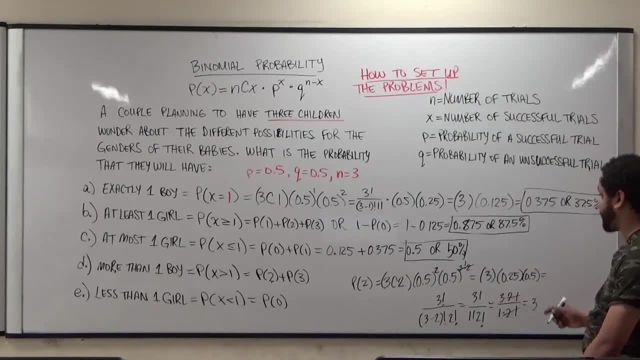 And this again becomes All we have to do is multiply this with our calculator. We see, we'll get the same result we did with this line, because 3 times 0.125 gives us 0.375.. So our first probability here is 0.375.. 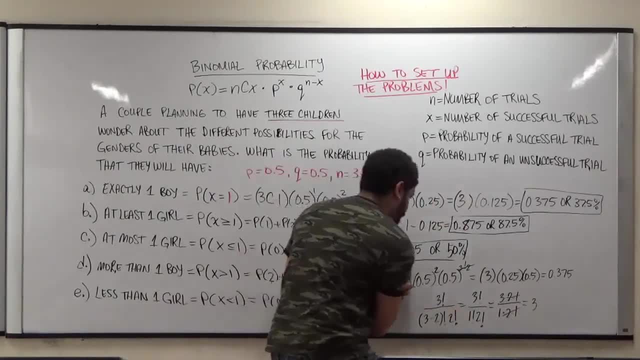 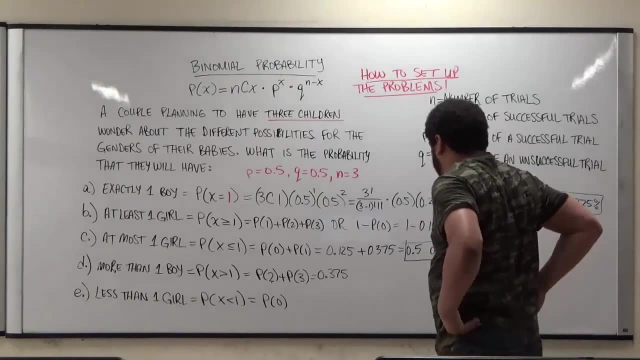 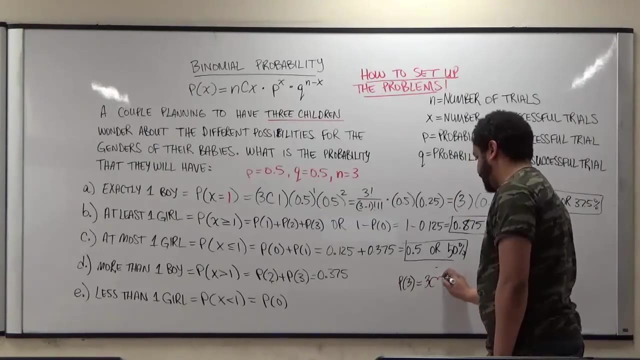 And we can wash off the sample space we have here And we'll do the second component now. So for the second component we're doing the probability of 2.. 3 boys, So that's going to be 3 combination, 3.. 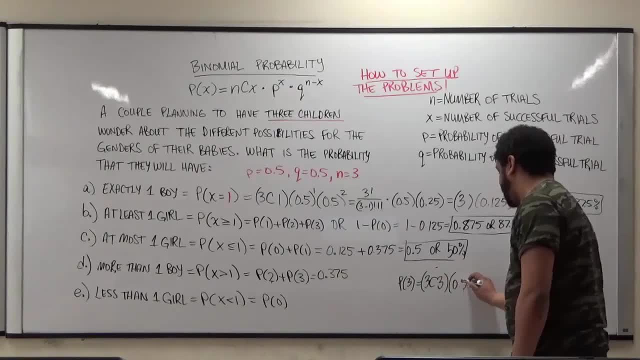 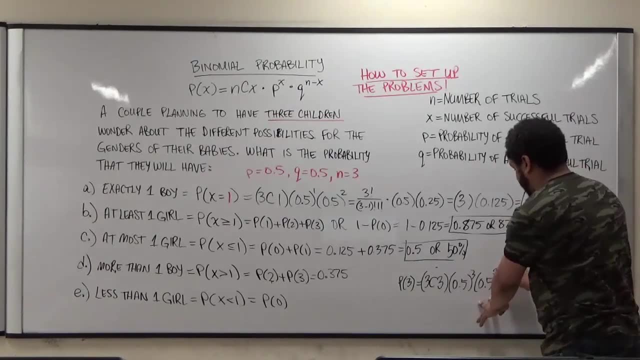 We're multiplying this by 0.5 to the power of 3 times the power of 0.5, of 0.5 to the power of 3, take away 3, which is 0. So this becomes 1.. 3 combination, 3.. 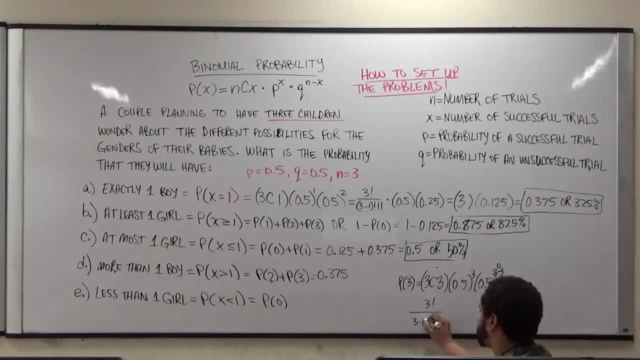 Let's take a look at it: 3 minus 3 factorial times 3 factorial, 3 minus 3 is 0.. So we have 3 factorial over 0 factorial and 3 factorial, 0 factorial is 1.. 3 divides 3 evenly, because they're the same factorial. 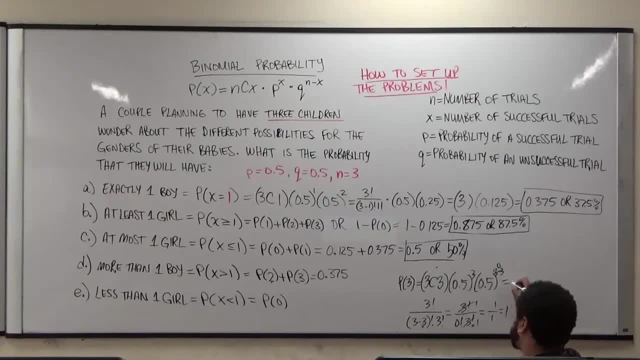 We get 1 and 1.. So we have 1 over. 1 is just 1.. So the 3 combination 3 is 1.. And we have 0.5 to the third power is 0.125.. 0.5 to the power of 0 is just 1.. 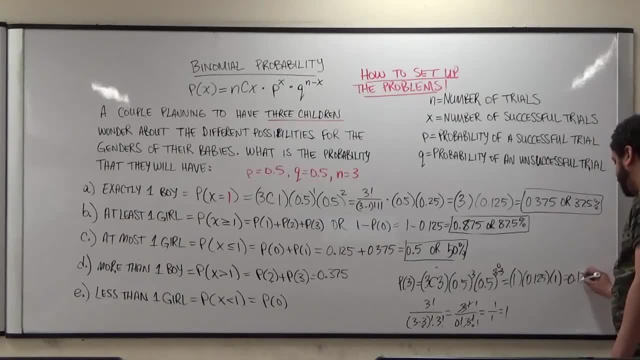 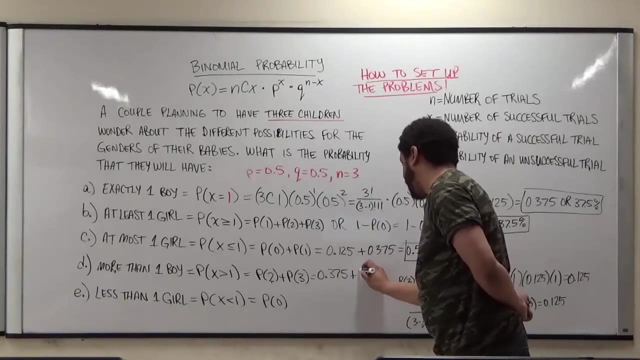 And that becomes 0.125.. And now this 0.125 is the probability of 3.. So the P3 is 0.125.. And we're adding this to the probability of 2, which is 0.3275.. 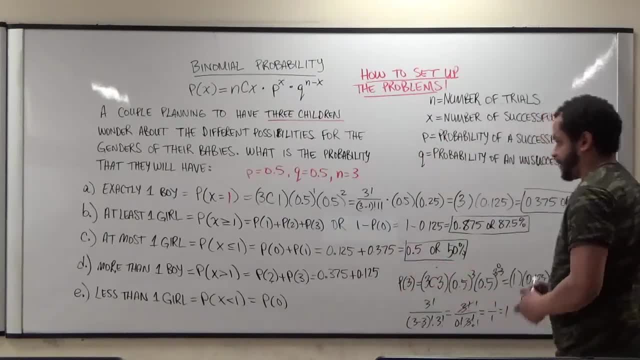 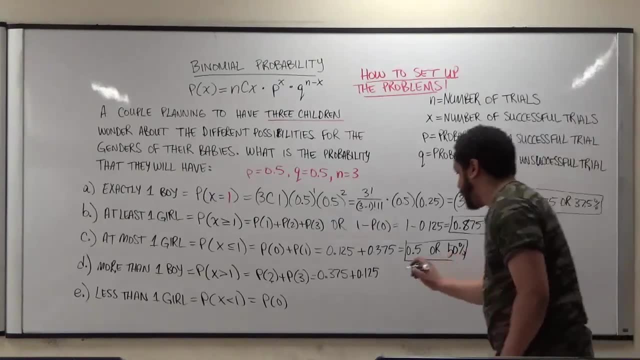 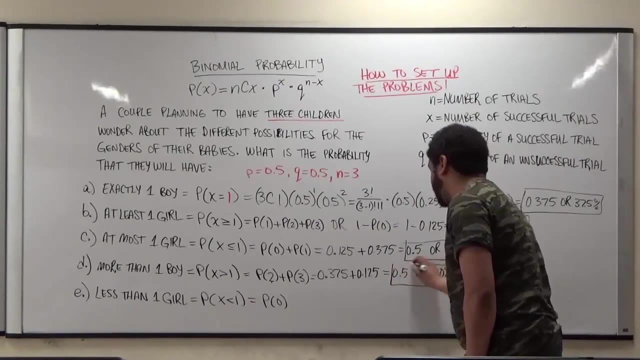 So this plus this is the same result we got for the last problem, right. So this here also gives us 0.5. Or 50% again. And we can also think about this real quick right: More than 1 boy is having 2 boys or 3 boys. 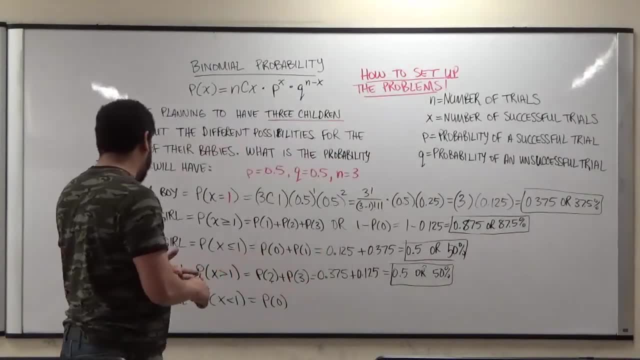 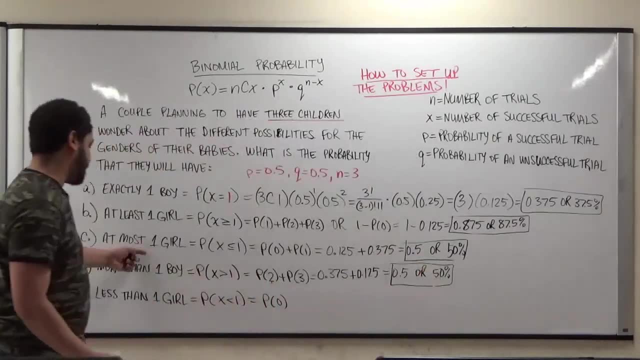 At most if we have 2 or 3 boys, that would be 50%. I think these are both complement events. if we look really closely, right At most 1 girl and more than 1 boy, They're actually complement events probably. 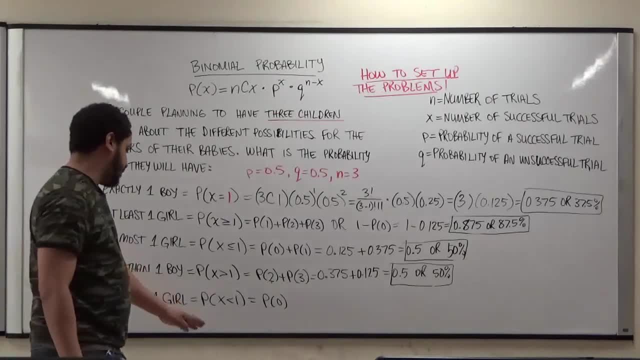 Looking, finally, at part E, here we have less than 1 girl, which is the probability of 0.. And we've done this probability today already, Because we did the at least 1 girl situation And we know the probability of having no girls is 0.125. 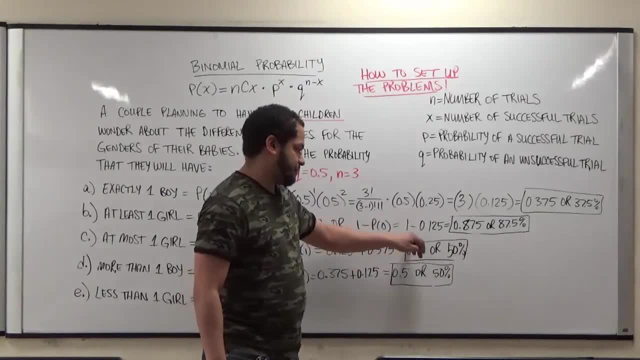 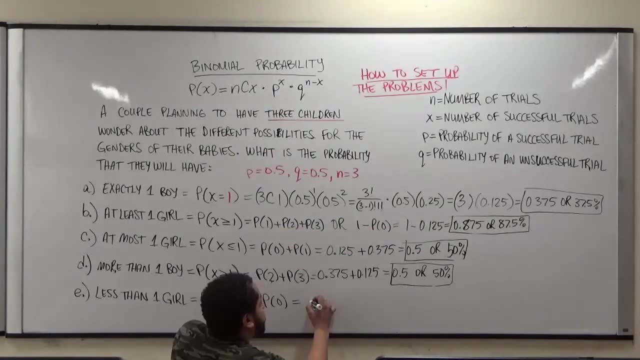 Because here we see it's 1 minus the probability of 0. And here we have 1 minus the 0.125.. We previously just did this for part B, So the solution for the last one is the same work we did for part B. 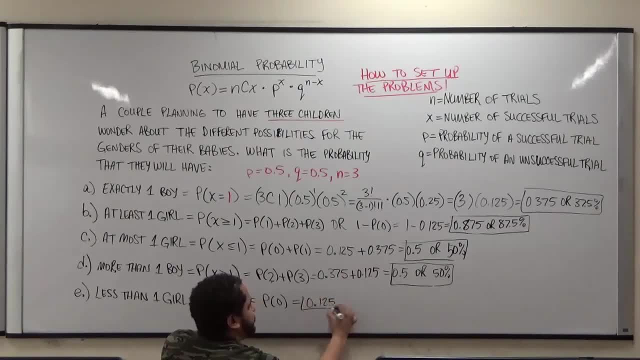 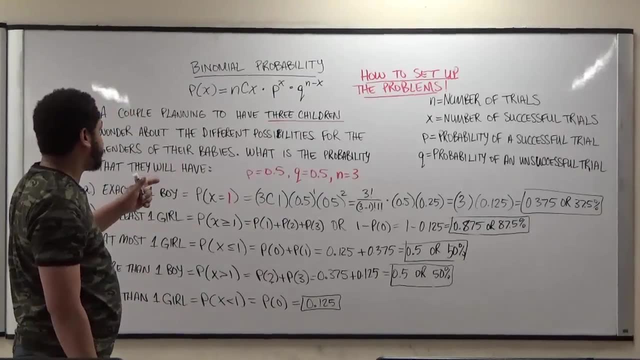 with the P of 0, which is 0.125.. So remember, when you're doing these binomial probability distributions, make sure it meets the four requirements. After you check it meets the four requirements, set up your problems first by taking your words. 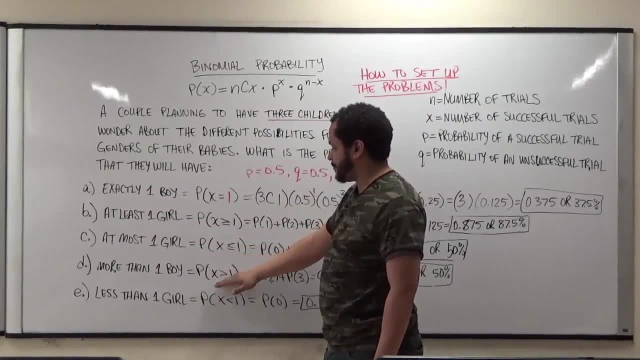 translating them into probability functions And once you do the functions, complete them out and solve them from there. alright, Thank you.